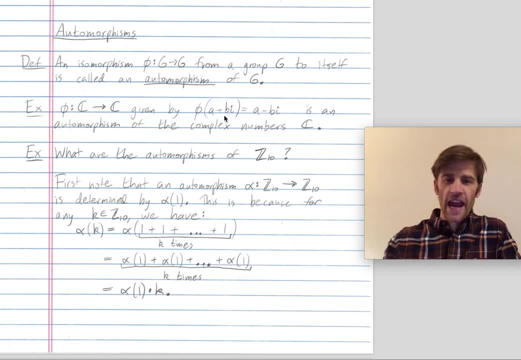 An automorphism is you can map the complex number a plus bi, where i is the square root of negative 1, to its complex conjugate, a minus bi. And this is an automorphism. It preserves a group structure even though it's not the identity map. 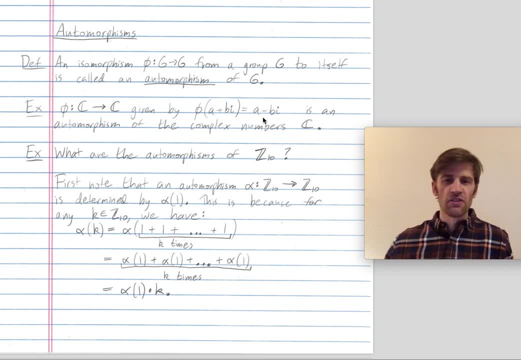 Okay, this video is just an introduction. So for the rest of this lecture, we'll focus on what are the automorphisms of Z mod 10. 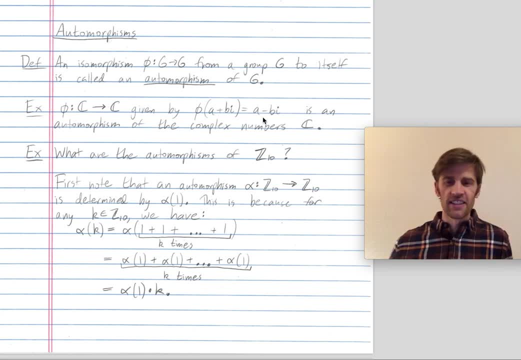 So this is the number 0 up through 9. Addition is our operation mod 10. What we'll be saying here will really hold for any cyclic group Z mod n, but I'm using Z 10 as a specific example. 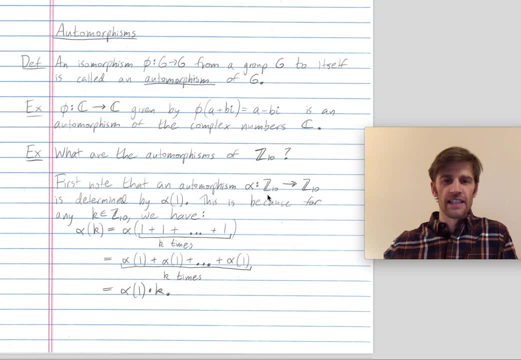 So let's say alpha is an automorphism from Z 10 to itself. One comment is that the entire map alpha is determined by alpha of 1. If I tell you where alpha maps 1, then you know where alpha maps any other element. This is because 1 is a generator, as you'll see. So let's say I tell you where alpha of 1 maps. It maps to alpha of 1. Well, where does alpha map k? So k is an arbitrary element of Z 10. Well, note that alpha of k is just alpha of 1. 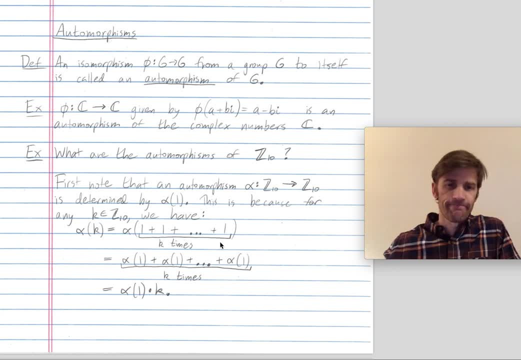 And now, using the property that alpha is an automorphism, or more generally an isomorphism, we know that alpha of a bunch of things combined together is alpha of each individual thing then all combined together. That's the defining property of an isomorphism. 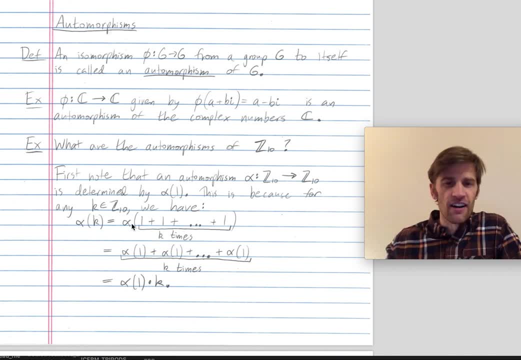 So alpha of 1 plus 1 plus 1 plus 1 is just alpha of 1 plus alpha of 1 plus dot dot dot plus alpha of 1, since alpha is an automorphism, or more generally an isomorphism, hence preserves the group structure. 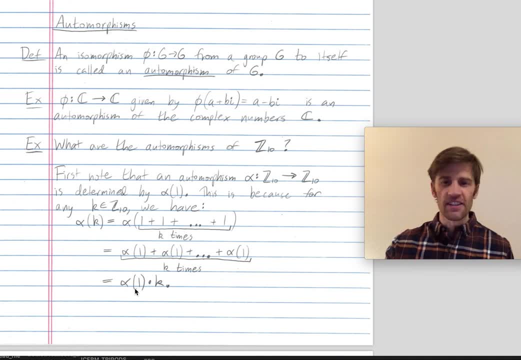 And anything added to itself k times is just alpha of 1 times k. So where does alpha map k? It maps it to k times alpha of 1. 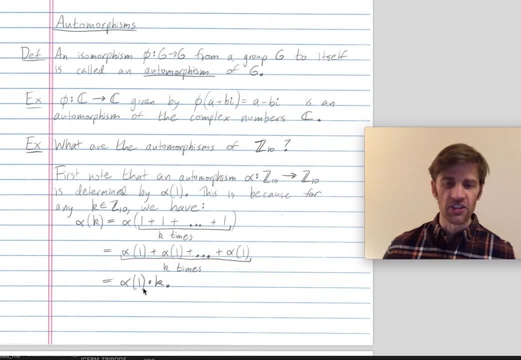 That's the sense in which where alpha maps 1 determines where alpha maps anything. You know, if alpha maps 1 to 7, then alpha maps k to 7 times k. Fantastic. All right. 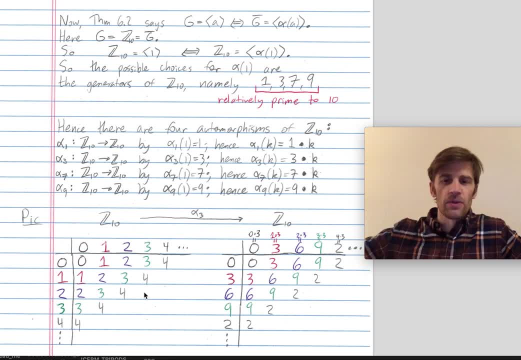 So in our previous lecture, we talked about properties of isomorphism. And one property was that if two groups were isomorphic, and if both groups were cyclic, then a generator of the first group had to map to a generator of the second group. 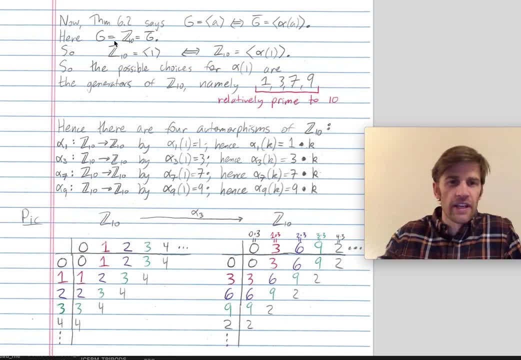 Here, we're in the case where we're looking at automorphisms. So our first group and our second group are the same, Z mod 10. 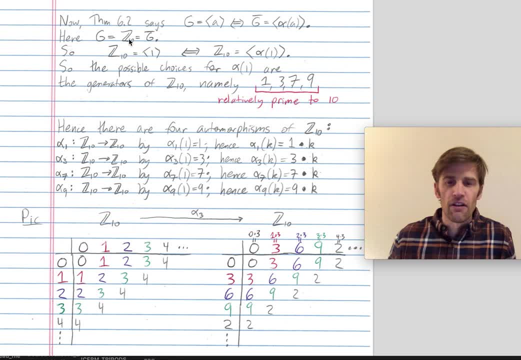 So we're mapping Z mod 10 to itself. And so here, what we're doing is we're mapping it to itself. what this property says is a generator of Z10 under an automorphism alpha has to get mapped to another generator of Z10. That's what this third line says here. Since 1 is a generator of Z10, it has to be the case that where 1 gets mapped also has to be a generator of Z10. And we know the generators of Z10, they're the numbers relatively prime to 10. So they're 1, 3, 7, and 9. So this is telling us that under our automorphism, 1 has to get mapped to a generator of Z10. So 1 has to get mapped to 1, 3, 7, or 9, another generator. So there's only four automorphisms from Z10 to itself. Let's call them alpha 1, alpha 3, alpha 7, and alpha 9, depending on where the generator 1 gets mapped. 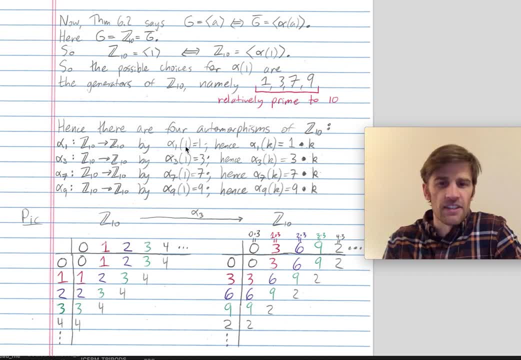 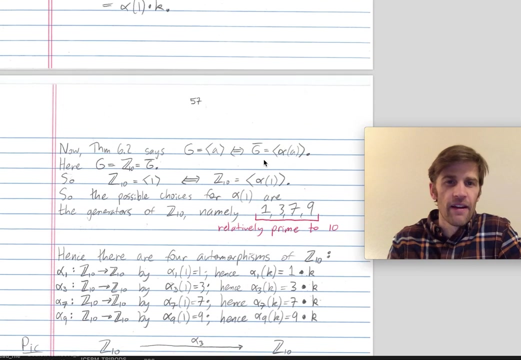 So alpha 1 maps the generator 1 to 1. Alpha 3 is going to map the generator 1 to 3. Alpha 7 is going to map 1 to 7. And alpha 9 is going to map 1 to 9. More generally, where do each of these automorphisms, alpha 1, 3, 7, and 9, map an arbitrary input K? Well, that's what we learned up above. Where alpha maps K? 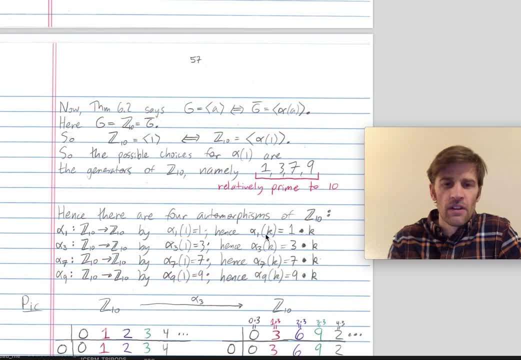 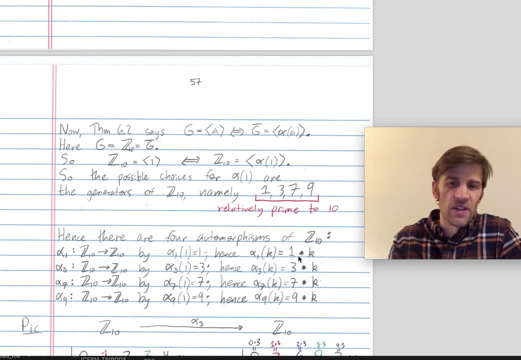 It's just K times where alpha maps 1. So since alpha 1 maps 1 to 1, alpha 1 maps K to have 1 times K, and et cetera. So alpha 7 is going to be this automorphism that maps any input 7, sorry, any input K to 7 times K. And alpha 9 is going to be an automorphism that maps any input K to 9 times K. 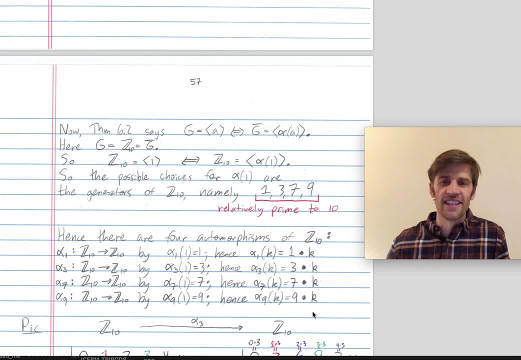 This is a complete list of all automorphisms of Z10. Any other automorphism you write down is going to be a map that's equal on the nose to one of these four right here. 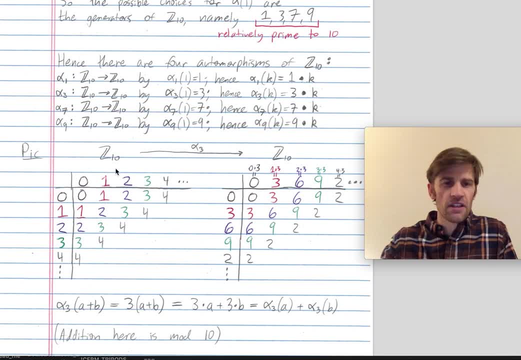 Let me draw a picture of this map, alpha 3. So on the left, we have part of the multiplication table for Z10, or Cayley table for Z10. 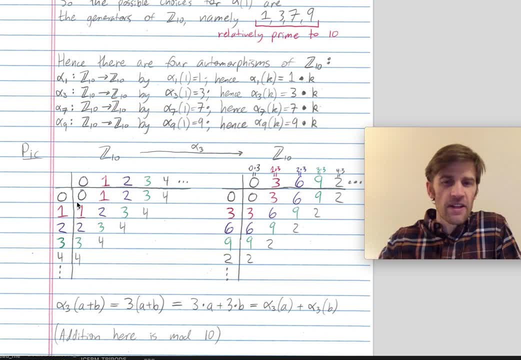 If you drew colors for each different element and you filled out this entire Cayley table, we'd have these diagonal stripes because this is a cyclic group. And alpha 3 is going to map each element K to just 3 times K. So 0 maps to 0, 1 maps to 3, 2 maps to 6, 3 maps to 9, 4 maps to 4 times 3, which is 12, but mod 10, that's 2. So alpha 3 is going to map each element K to just 3 times K. So alpha 3 is going to map each element K to just 2, et cetera. 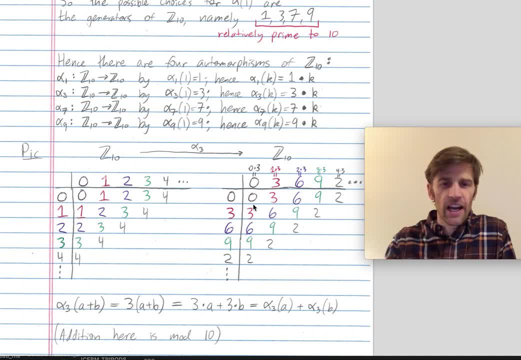 And you'll notice that on the right hand side, we still have the same diagonal stripes. 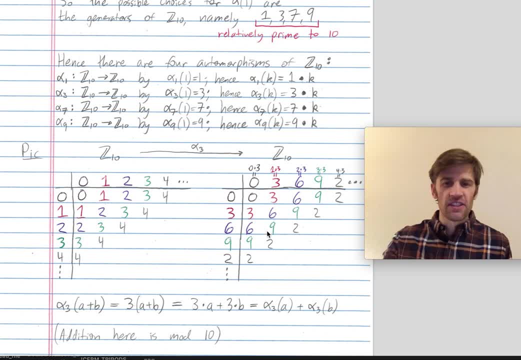 Okay? So you can see that these two groups are isomorphic because the patterns of their Cayley tables as preserved. But this is not the identity map, right? Every element is being multiplied by 3.